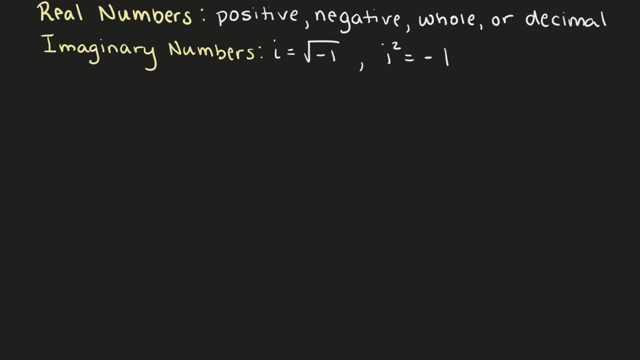 So we know what real numbers look like. This can be any number like 2, negative 5, 12.7, negative 30.234.. These are all real numbers. Let's look at some examples of imaginary numbers. Say we have the square root of negative 64.. 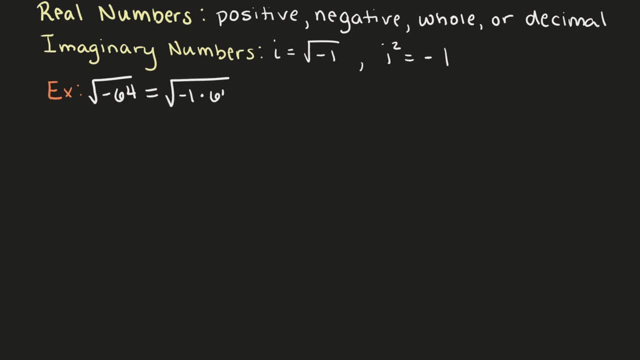 Well, this is the same as the square root of negative 1 times 64. So we can break that up and that gives us the square root of negative 1 times the square root of 64. And our number becomes 8i, where i represents the square root of negative 1.. 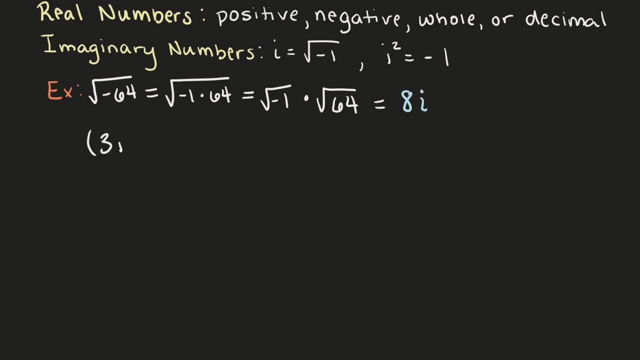 Let's take 3i raised to the second power or 3i squared. Well, we can distribute our exponent and get 3 squared times i squared, which gives us 9i squared. i squared is equal to the square root of negative 1 times 64.. 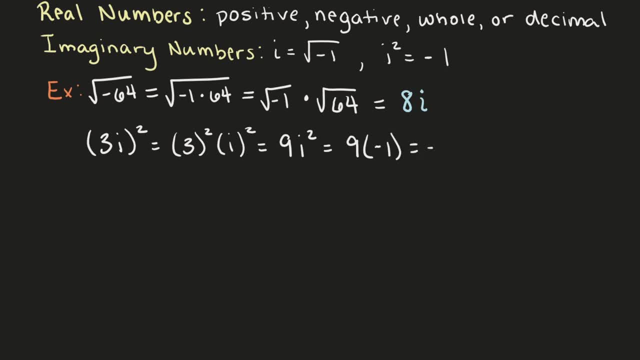 i squared is equal to negative 1, so we get 9 times negative 1,, which is negative 9.. So some examples of complex numbers would be negative 2 plus 4i, where negative 2 is your a and 4i is your bi term. 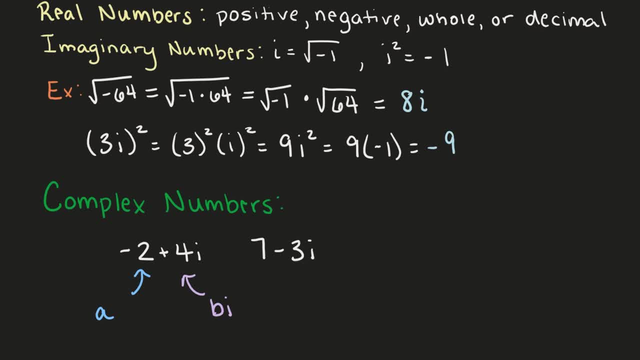 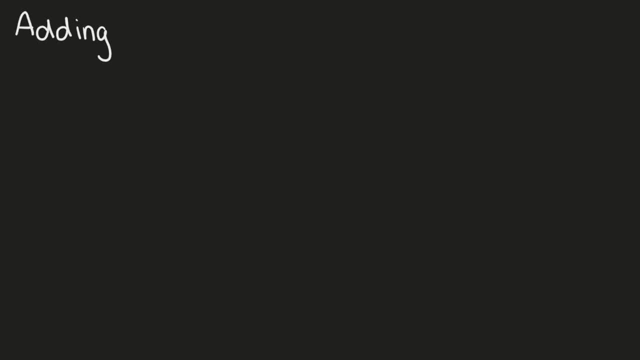 7 minus 3i and 12 plus 6i. Let's look at algebra. Let's start with adding complex numbers. Remember a complex number is the number in the form a plus bi. So say we're adding two complex numbers together. 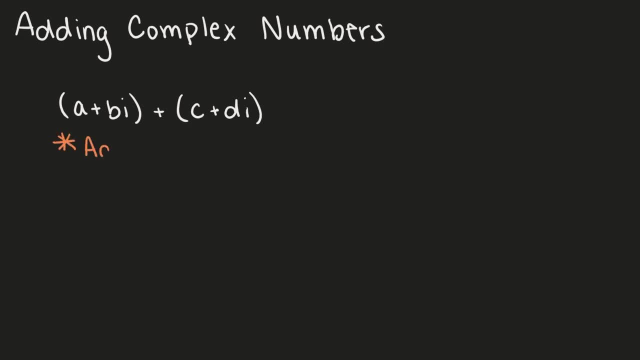 We have a plus bi, plus c plus di. All we need to do is add the like terms. So in this case we want to group our real numbers together and our imaginary numbers together. a and c are our real numbers and our like terms. 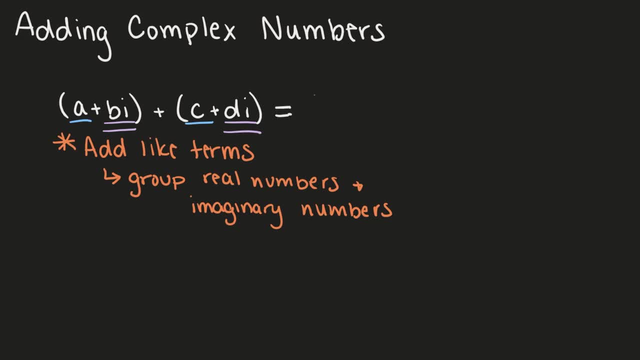 bi and di are imaginary numbers and are like terms, So we can rewrite this as a plus c plus bi plus di. Let's move into some examples. First, we have 3 plus 6i plus 4 minus 2i. 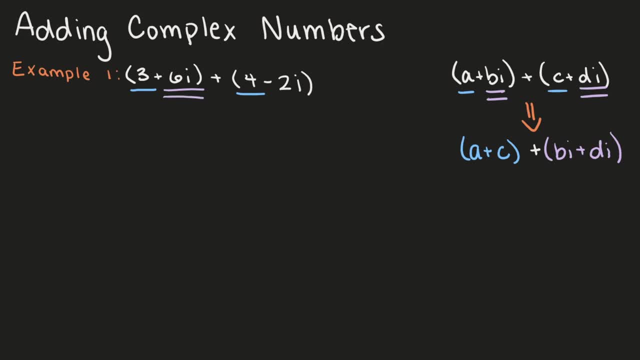 3 and 4 are our real numbers and our like terms, so we'll group those together. 6i and negative 2i are imaginary numbers and like terms and we'll group those together. That gives us 3 plus 4 plus 6i minus 2i. 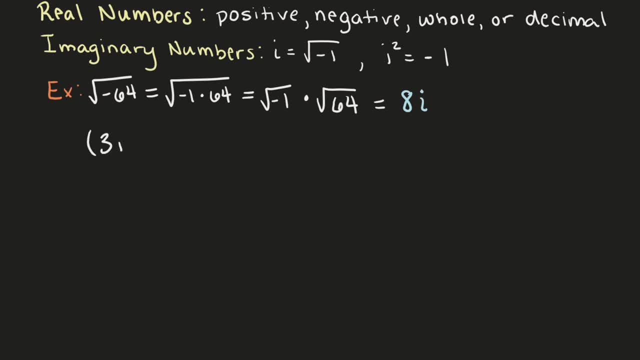 Lets take 3i raised to the 2nd power, or 3i squared. Well, we can distribute our exponent and get 3 squared times i squared, which gives us 9i squared. i squared is equal to 8i squared. 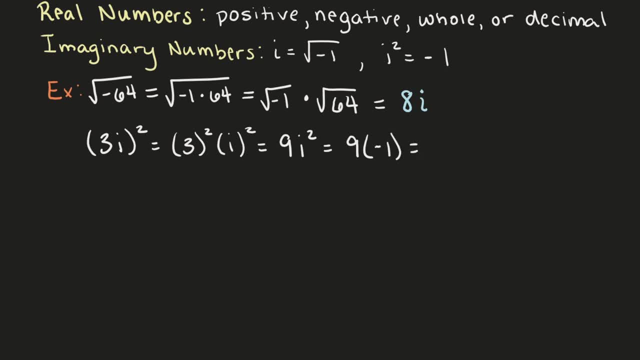 Let's do that again: equal to negative 1, so we get 9 times negative 1,, which is negative 9.. So some examples of complex numbers would be negative 2 plus 4i, where negative 2 is your a and 4i is your bi term, 7 minus 3i and 12 plus 6i. 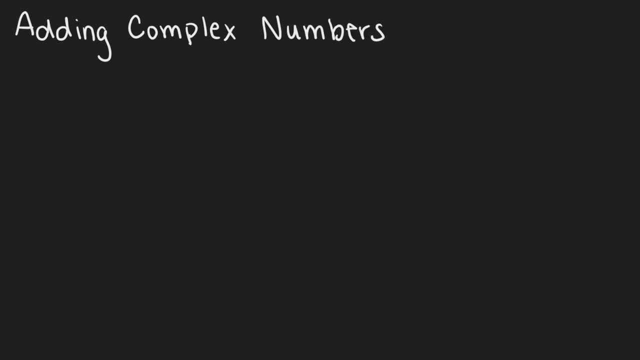 Let's look at adding complex numbers. Remember, a complex number is the number in the form a plus bi. So say we're adding two complex numbers together, We have a plus bi plus c plus di. All we need to do is add the like terms. 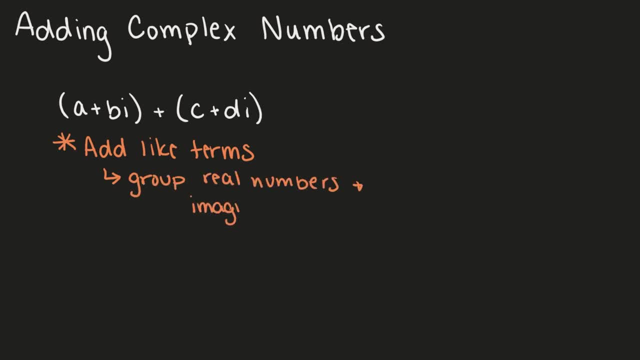 So in this case we want to group our real numbers together and our imaginary numbers together. a and c are our real numbers and our like terms. bi and di are our imaginary numbers and our like terms. So we can rewrite this as a plus c plus bi plus di. 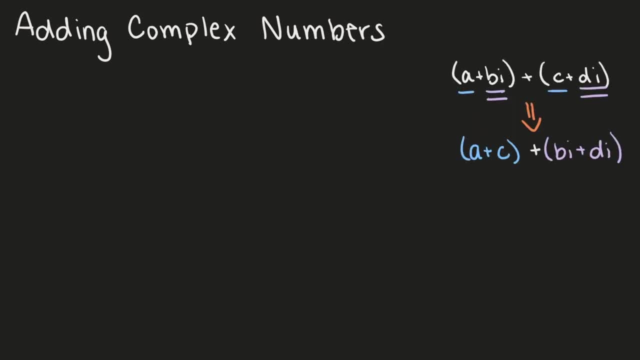 Let's move into some examples. First, we have 3 plus 6i plus 4 minus 2i. 3 and 4 are our real numbers and our like terms, so we'll group those together. 6i and negative 2i are imaginary numbers and like terms, and we'll group those together. 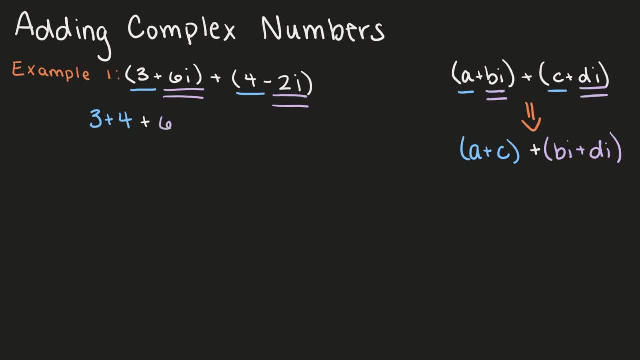 That gives us 3 plus 4 plus 6i minus 2i. Combining those gives us 7 plus 4i. Let's take another example. We have 5 plus 2 square root negative 16 plus 2 plus 3 square root negative 9.. 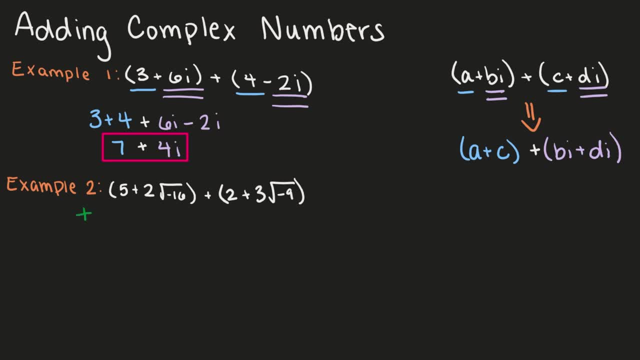 The first thing we want to do is rewrite both of these expressions as complex numbers. We can do that by modifying our real numbers. By the way, it's easy if you're familiar with the real numbers and using the algebra, because it's pretty easy. 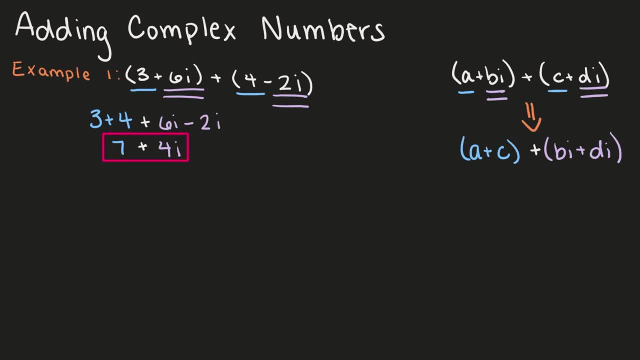 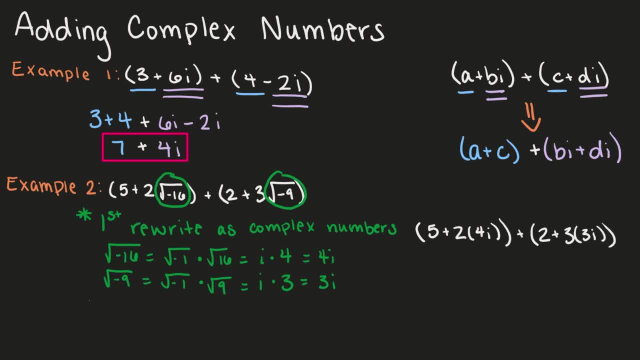 plus 4i plus 2 plus 3 times 3i. That makes our complex numbers 5 plus 8i plus 2 plus 9i. Our like terms are 5 and 2 and 8i and 9i. So 5 plus 2 gives us 7, 8i plus 9i gives us 17i, and our final answer is 7 plus 17i. 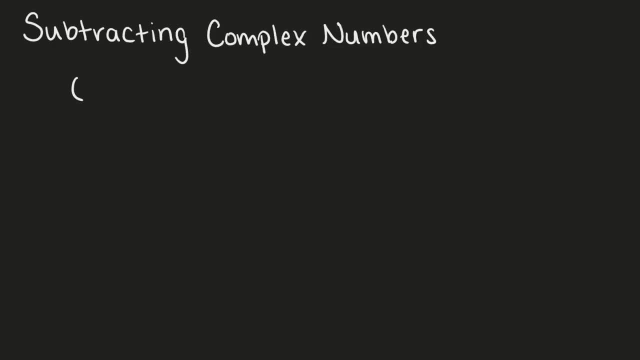 Next let's look at subtracting complex numbers. Subtracting complex numbers is just like adding them: We're going to combine our like terms, except, instead of adding our like terms, we're going to subtract our like terms. So, if we have a plus bi, minus c plus di, a and c are like terms, bi and di are like terms. 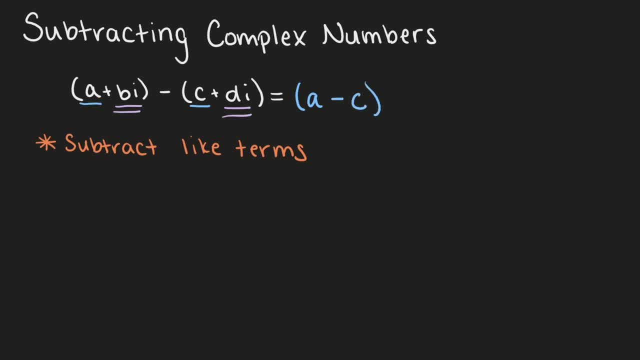 and our solution is going to be a minus c plus bi minus di. Let's look at some examples. Let's take the example nine minus six. i minus twelve plus two i. Nine and twelve are like terms, negative six, i and two i are also like terms. 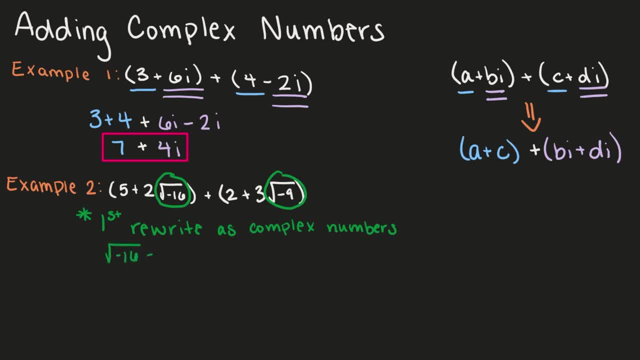 The first thing we want to do is to round the numbers. We're going to do a good job of doing so by just identifying our square root negative 16 and our square root negative 9.. The square root of negative 16 is equal to the square root of negative 1 times the square. 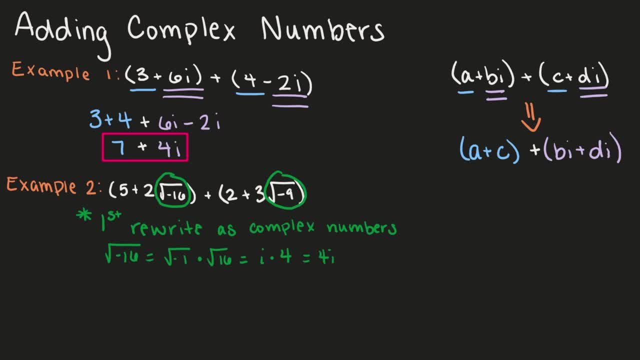 root of 16,, which is i times 4, or just 4i. The square root of negative 9 is equal to the square root of negative 1 times the square root of 9,, which is i times 3, and that equals 3i. 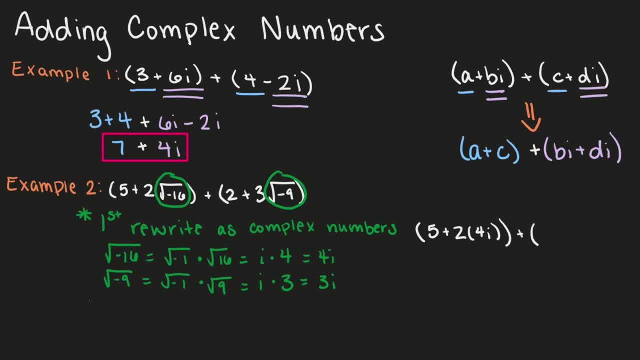 We can rewrite our expression as 3i plus 2i plus 4i plus 3i, 5 plus 2 times 4i plus 2 plus 3 times 3i. That makes our complex numbers 5 plus 8i plus 2 plus 9i. 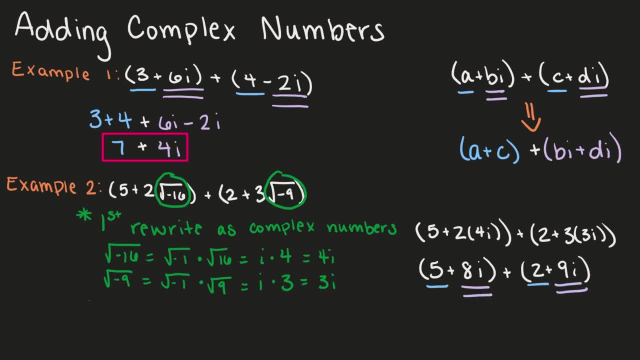 Our like terms are 5 and 2 and 8i and 9i. So 5 plus 2 gives us 7,, 8i plus 9i gives us 17i, and our final answer is 7 plus 17i. 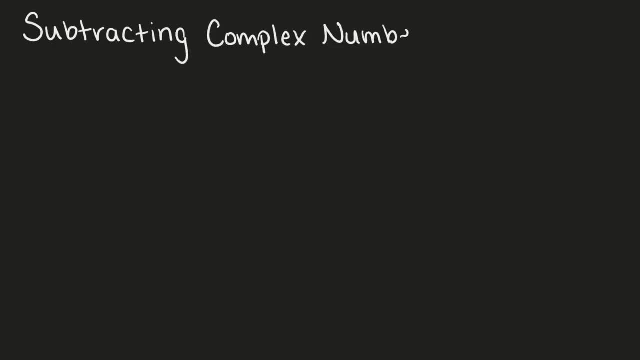 Next let's look at subtracting complex numbers. Subtracting complex numbers is just like adding them: We're going to combine our like terms, except, instead of adding our like terms, we're going to subtract our like terms. So, if we have a plus bi, minus c plus di, a and c are like terms, bi and di are like terms. 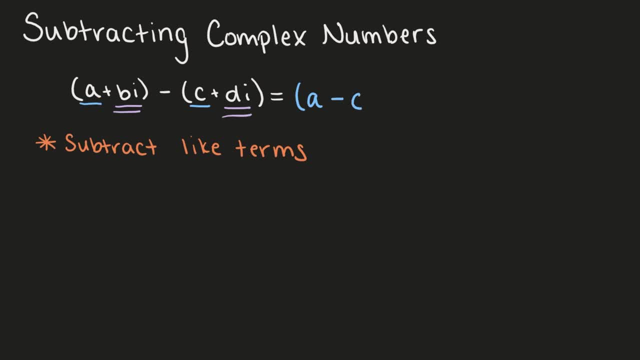 and our solution is going to be a minus c plus di. So we have a minus c plus bi minus di. Let's look at some examples. Let's take the example 9 minus 6i minus 12 plus 2i. 9 and 12 are like terms, negative 6i and 2i are also like terms, so we'll group those. 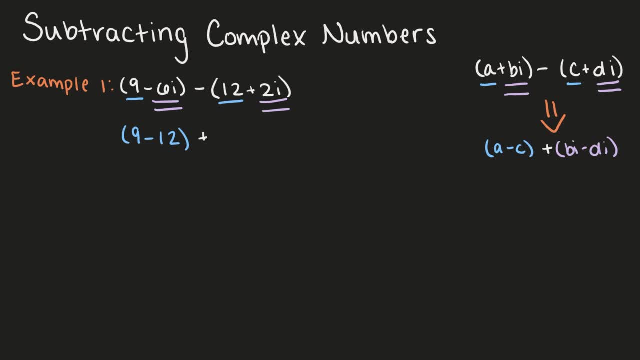 We have 9 minus 12 plus negative 6i minus 2i. That gives us negative 3 plus negative 8i. Let's take another example: We have 3 minus 2 times the square root of negative, 18 minus 2 plus 3 times the square root of negative 8.. 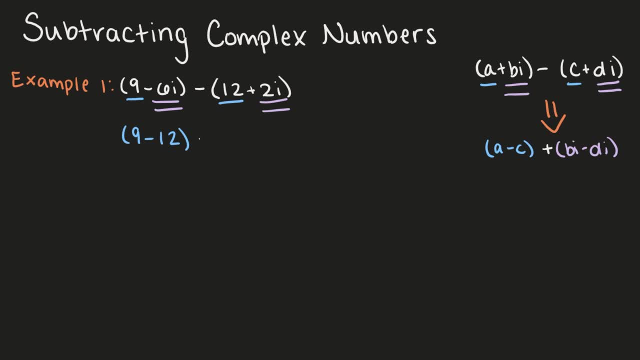 So we'll group those. We have nine minus twelve plus negative six i minus two i. Negative six i minus two i. That gives us negative three plus negative eight i. Let's take another example: We have three minus two- times the square root of negative. eighteen minus two plus three. 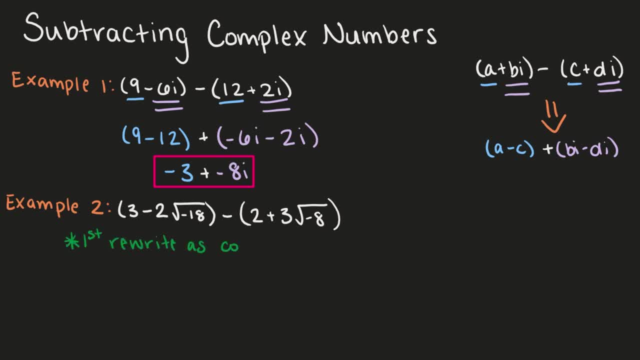 times the square root of negative eight. The first thing we want to do is rewrite these expressions as complex numbers, So let's start with the square root of negative eighteen. Well, this is equal to the square root of negative one times the square root of eighteen. 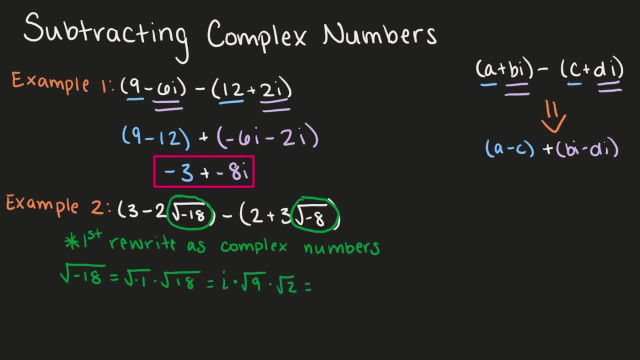 The square root of negative one becomes i times the square root of nine times the square root of two. Nine is a perfect square, so that gives us three. i square root two. The square root of negative eight can be written as the square root of negative one times the. 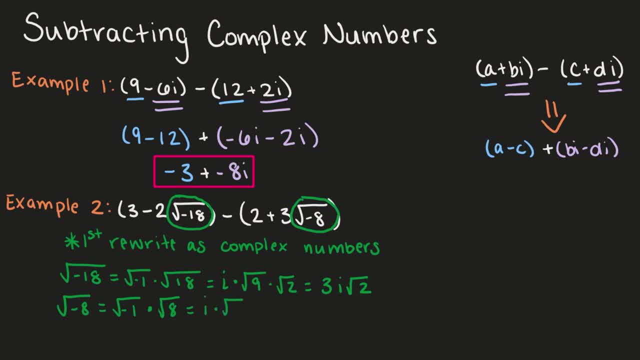 square root of eight, Which is i, times the square root of four, So that gives us three. i square root two. The square root of negative eight can be written as the square root of negative one times the square root of four, which is a perfect square, times the square root of two, which becomes 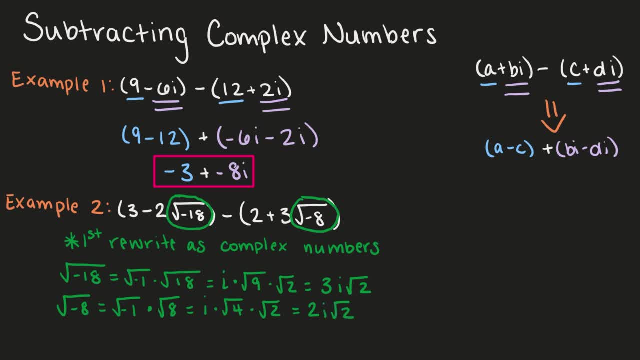 two i square root two. Let's rewrite our expressions using the imaginary numbers we just found. That gives us three minus six i square root two minus two plus six i square root two. Three and two are like terms And negative. six i square root two and six i square root two are also like terms for. 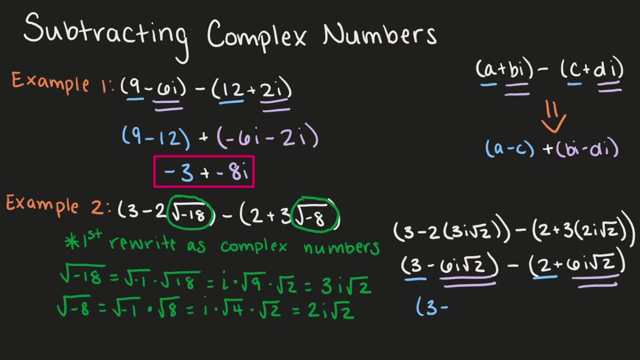 two reasons. They are both imaginary numbers and they both have a square root two, which means they can be combined. Subtracting our like terms gives us a final answer of one plus negative twelve. i square root two. Now let's look at multiplying complex numbers. 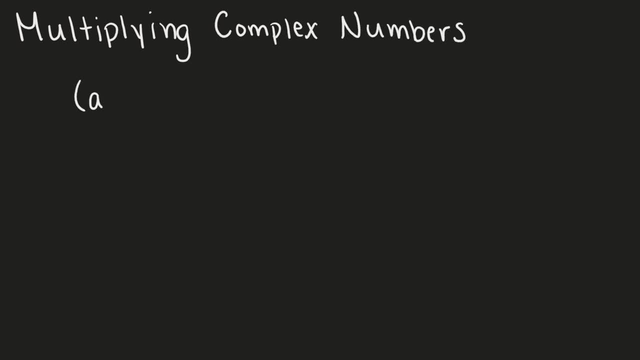 To multiply complex numbers we use the FOIL method. FOIL method is simply first, outside, inside last. The word FOIL corresponds to which terms we are multiplying. So if we have a plus bi times c plus di, we'll multiply the first terms, which is a times. 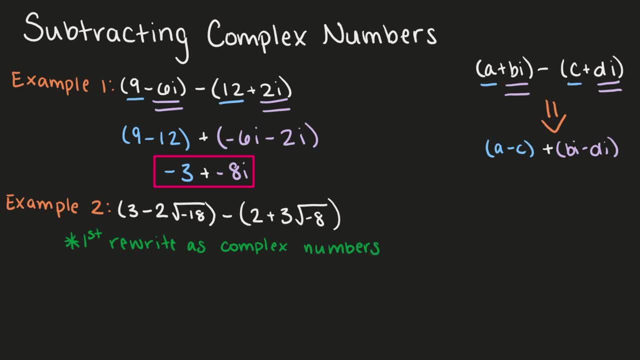 The first thing we want to do is rewrite these expressions as complex numbers. So let's start with the square root of negative 18.. So let's start with the square root of negative 18.. Well, this is equal to the square root of negative 1 times the square root of 18.. 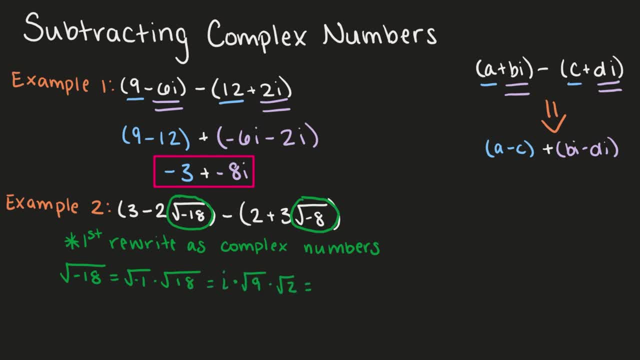 The square root of negative 1 becomes i times the square root of 9 times the square root of 2.. 9 is a perfect square, so that gives us 3i square root 2.. The square root of negative 8 can be written as the square root of negative 1 times the square root of 8,. 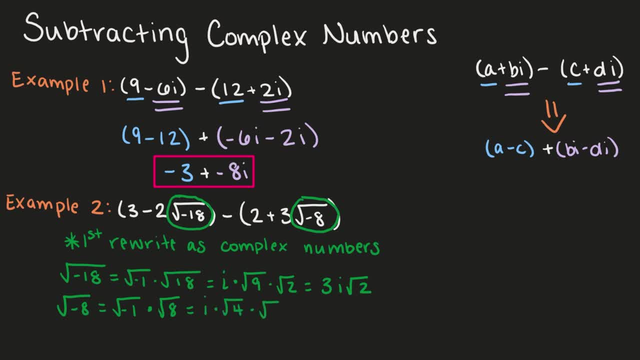 which is i, times the square root of 4,, which is a perfect square, times the square root of negative 8.. of 2,, which becomes 2i, square root 2.. Let's rewrite our expressions using the imaginary numbers we just found. 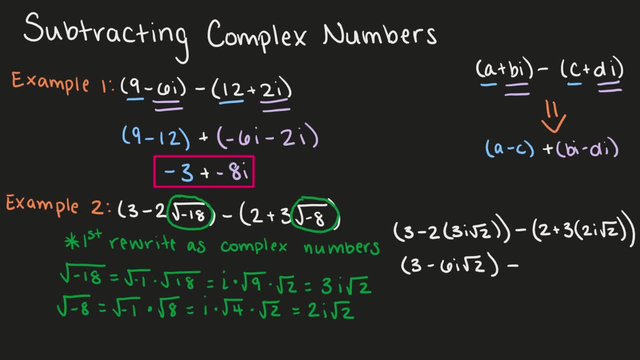 That gives us 3 minus 6i square root, 2 minus 2 plus 6i square root 2.. 3 and 2 are like terms and negative. 6i square root 2 and 6i square root 2 are also like terms for two reasons. 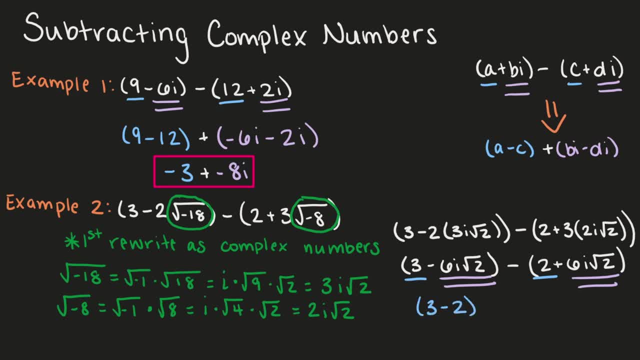 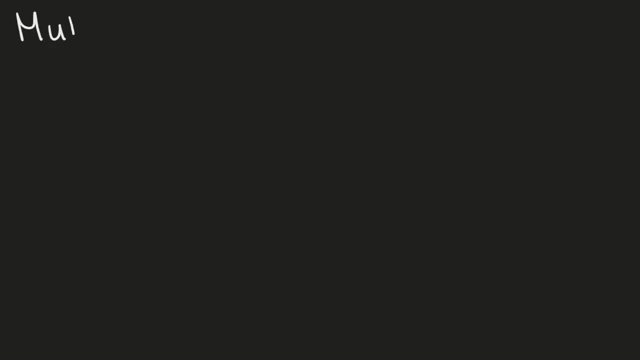 They are both imaginary numbers and they both have a square root 2, which means they can be combined. Subtracting our like terms gives us a final answer of 1 plus negative 12i, square root 2.. Now let's look at multiplying complex numbers. To multiply complex numbers, we use the FOIL. 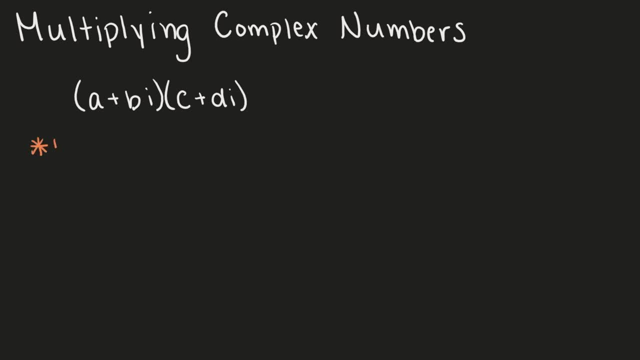 method. The FOIL method is simply first, outside, inside, last. The word FOIL corresponds to which terms we are multiplying. So if we have a plus bi times c plus di, we'll multiply the first terms, which is a times. 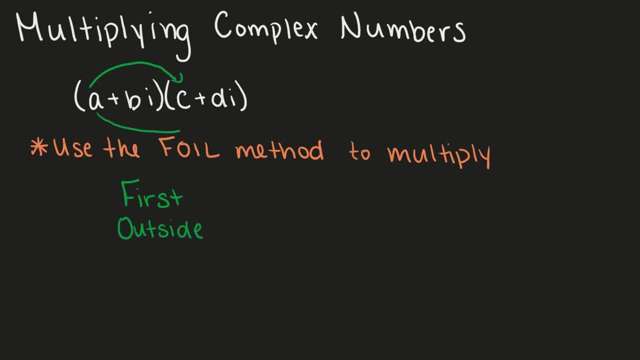 c, then the outside terms, which is a times di, the inside terms, which is bi times c, and the last terms, which is bi times di. This becomes ac plus adi plus bci plus bdi. squared- Keep in mind i squared is equal to the square root of negative 1 squared, which is negative 1.. 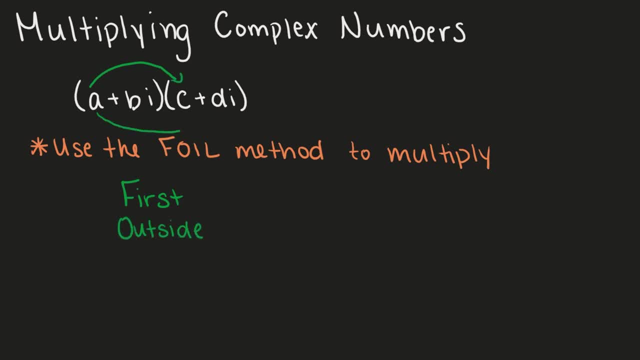 c, then the outside terms, which is a times di, the inside terms, which is bi times c, and the last terms, which is bi times di. This becomes ac plus adi plus bci plus bdi. squared, Keep in mind i, squared is equal to the square root of negative, one squared which is negative. 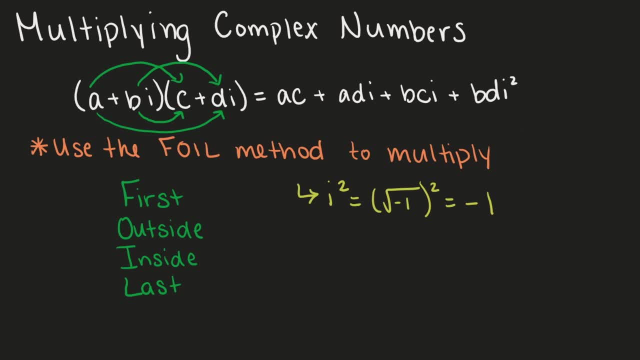 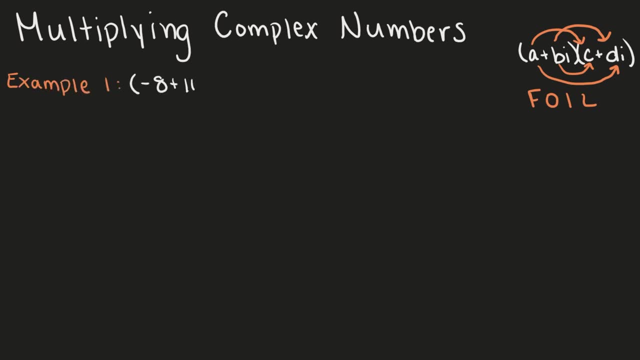 one. Now that we know how to multiply complex numbers using the FOIL method, let's look at a couple examples. First we have, First we have We have negative: eight plus ten. i times three plus eight. i. We'll multiply first outside, inside and last. 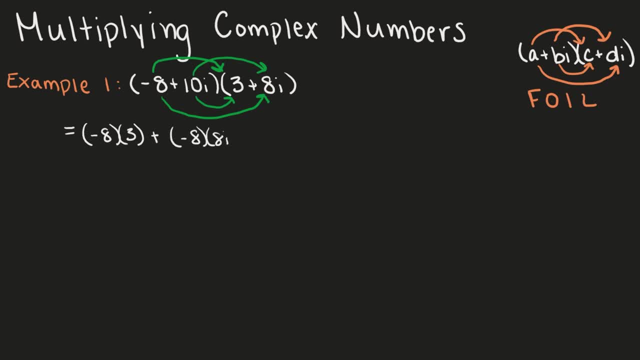 That gives us negative eight times three, plus negative eight times eight. i plus ten i times three plus ten i times eight i. This equals negative 24 minus 64, i plus 30, i plus 80, i squared, Remember, i squared. 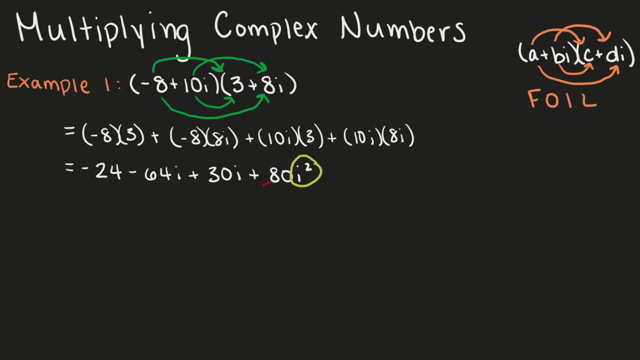 squared is the same as negative 1, so 80i squared becomes negative 80, and now we can identify our like terms. Negative 24 and negative 80 are like terms, and negative 64i and 30i are like terms. Combining these gives us our final. 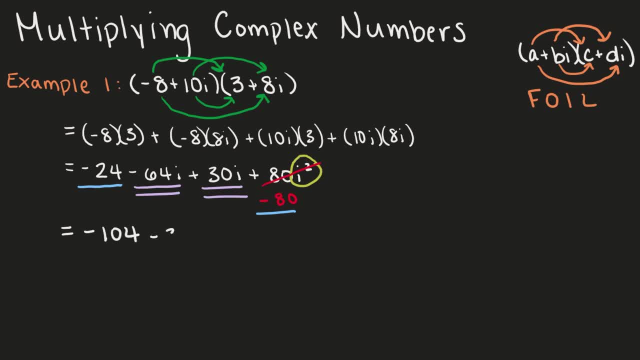 answer of negative 104 minus 34i. Let's take another example. We have 8 plus 7i times 4 plus 5i. Let's FOIL. so we multiply the first, outside, inside and last, and we get 8. 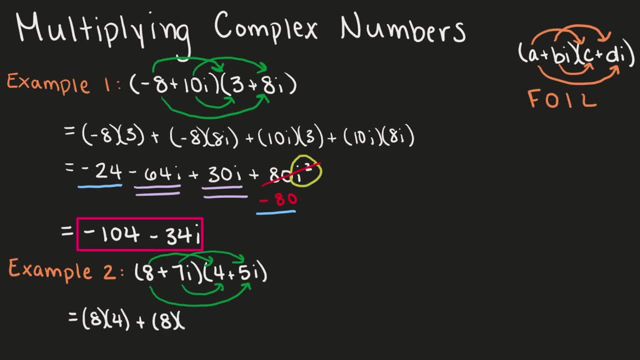 times 4 plus 8 times 5i plus 7i times 4 plus 7i times 5i. This gives us 32 plus 40i plus plus 28i plus 35i squared. Our i squared is negative 1, so that becomes negative 35. Identify. 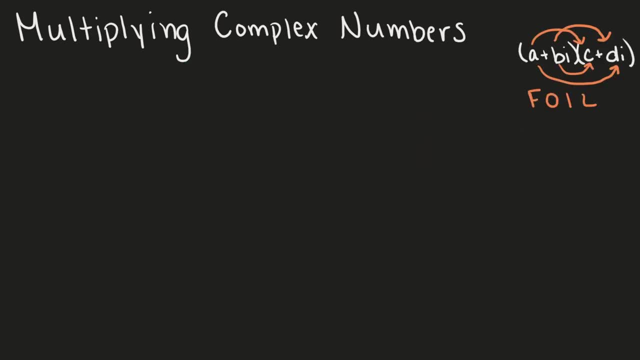 Now that we know how to multiply complex numbers using the FOIL method, let's look at a couple examples. First, we have negative 8 plus 10i times 3 plus 8i. We'll multiply first outside, inside and last. That gives us negative 8 times 3 plus negative 8 times 8i plus 10i times 3 plus 10i times 8i. 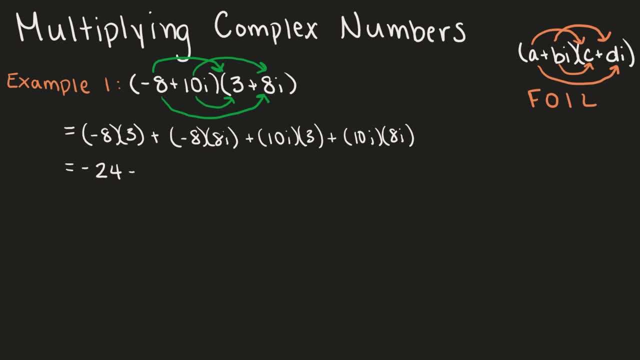 This equals negative 24 minus 64i plus 30i plus 80i squared. Remember i squared is the same as negative 1, so 80i squared becomes negative 1.. And now we can identify our like terms: Negative 24 and negative 80 are like terms, and negative 64i and 30i are like terms. 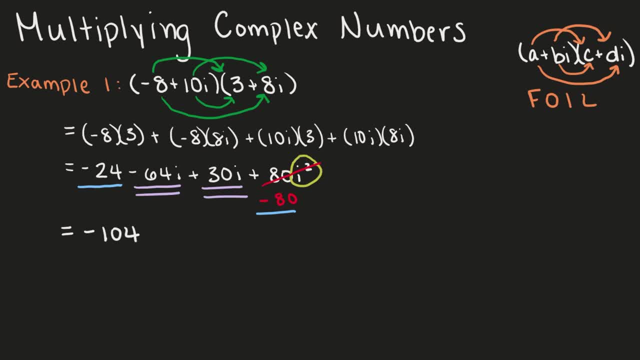 Combining these gives us our final answer of negative 104 minus 34i. Let's take another example. We have 8 plus 7i times 4 plus 5i. Let's FOIL. So we multiply the first outside, inside and last, and we get 8 times 4 plus 8 times 5i, plus 7i times 4 plus 7i times 5i. 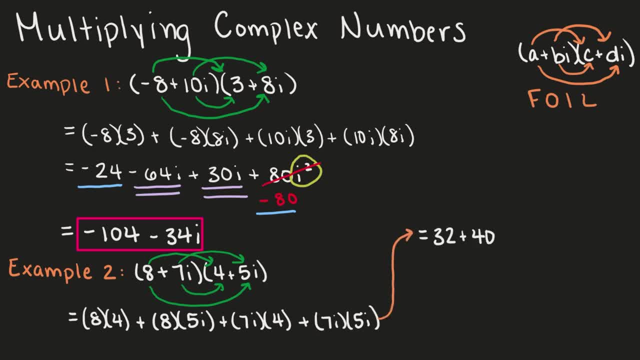 This gives us 32 plus 40i plus 28i plus 35i squared. Our i squared is negative 1, so that becomes negative 35.. We can identify and combine our like terms and we get negative 3 plus 68i. 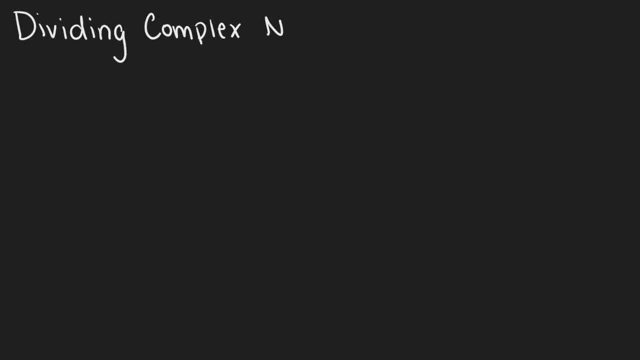 Finally, let's look at dividing complex numbers. A complex number division problem has the form a plus bi over c plus di. We use complex conjugates to divide complex numbers. You can find the complex conjugate by changing the sign of your complex number. 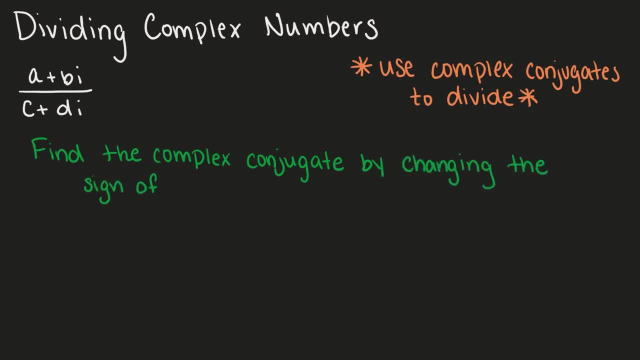 We're focused on the complex number in the denominator. This is because i is equal to the square root of negative 1, and we can't have square roots in our denominator. Our complex conjugate will allow us to remove any square roots from the denominator. 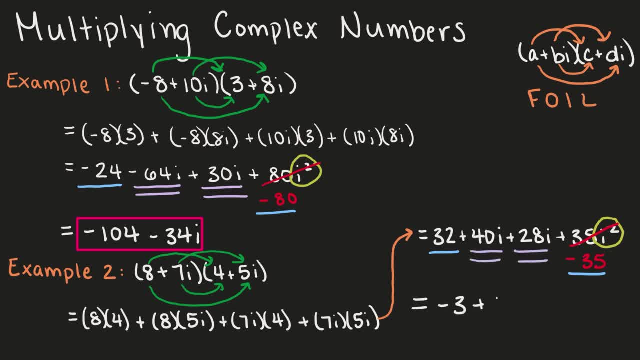 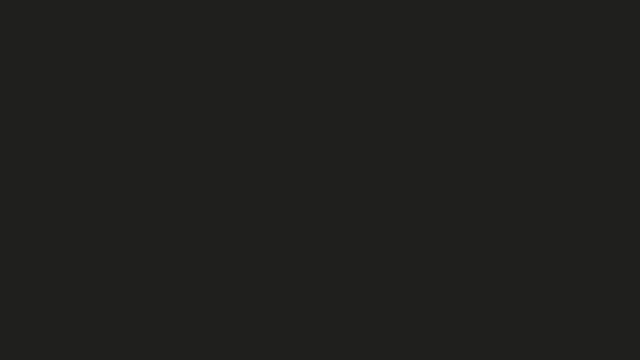 and combine our like terms and we get negative 3 plus 68i. Finally, let's look at dividing complex numbers. A complex number division problem has the form a plus bi over c plus di. We use complex conjugates to divide complex numbers. You can find the complex conjugate: 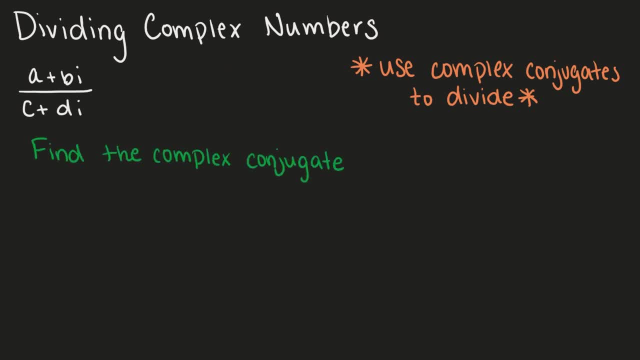 by changing the sign of your complex number. We're focused on the complex number in the denominator. This is because i is equal to the square root of negative 1, so dx is a definite integral of the denominator. We will work this out. and we can't have square roots in our denominator. Our complex conjugate will: 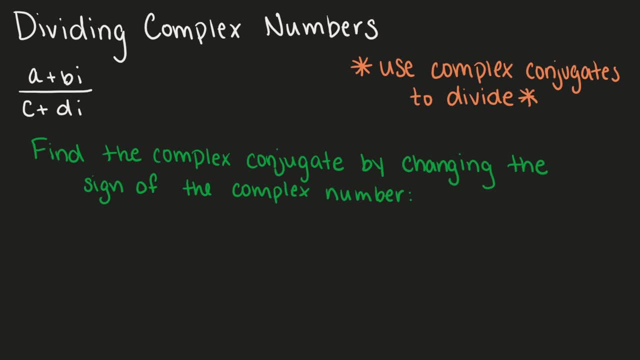 allow us to remove any square roots from the denominator. For example, a plus bi becomes a minus bi and vice versa, a minus bi becomes a plus bi. So when I multiply my complex number by my complex conjugate using the FOIL method, I get a. 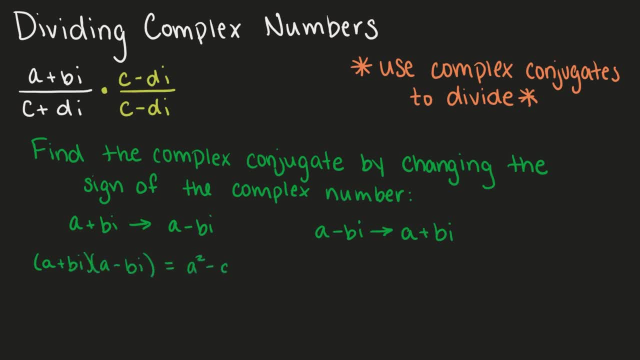 squared plus b squared. Regardless if it's a plus bi and the conjugate is a minus bi, or a minus bi and the conjugate is a plus bi, my product is always a squared plus b squared, which is my new denominator for my expression, which is: 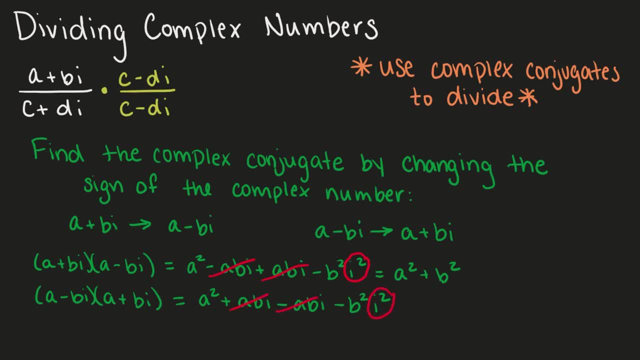 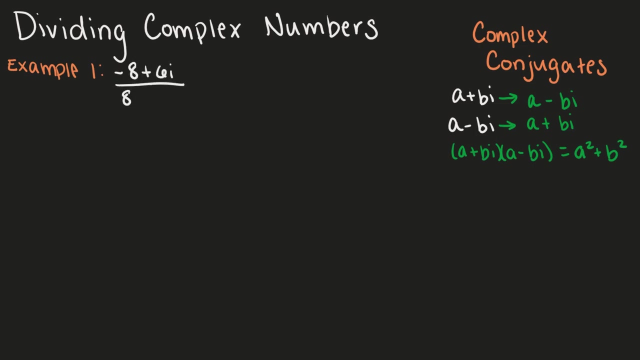 now valid because it is a real number. Let's look at this in action. We have negative 8 plus 6i divided by 8 minus 5i. Our complex conjugate is 8 plus 5i. We use the opposite sign of the complex. 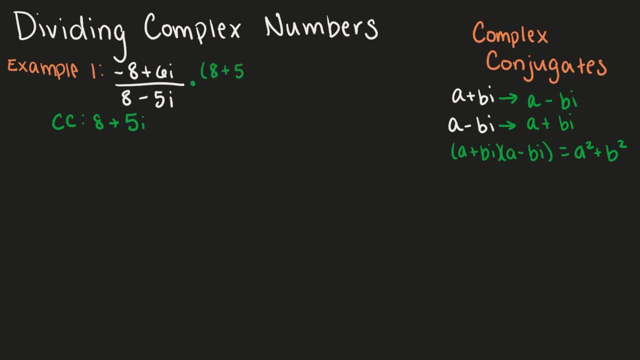 number in our denominator. So we're going to multiply top and bottom of this fraction by our complex conjugate, which is 8 plus 5i. We can always multiply any fraction by the same number over itself, because 8 plus 5i. 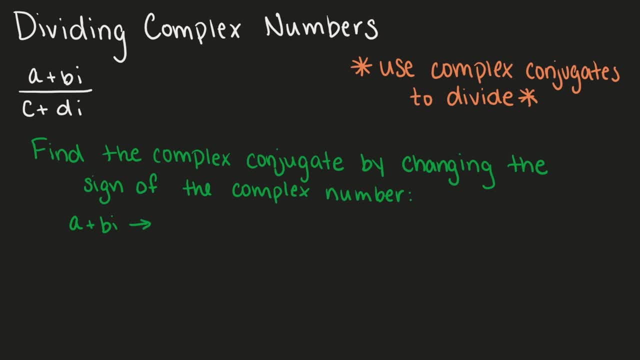 For example, a plus bi becomes a minus bi and vice versa, a minus bi becomes a plus bi. So when I multiply my complex number by my complex conjugate using the FOIL method, I get a squared plus b squared, Regardless if. 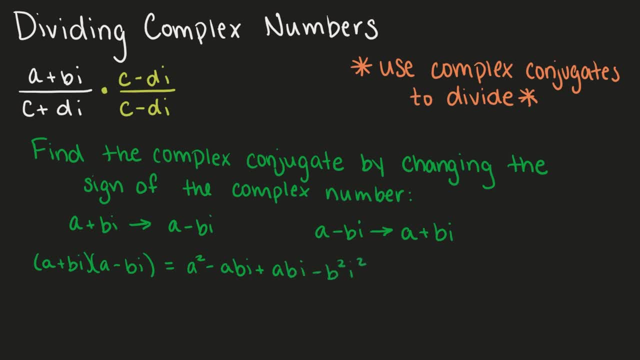 it's a plus bi and the conjugate is a minus bi, or a minus bi and the conjugate is a plus bi. my product is always a squared plus b squared, which is my new denominator for my expression, which is now valid because it is a real number. 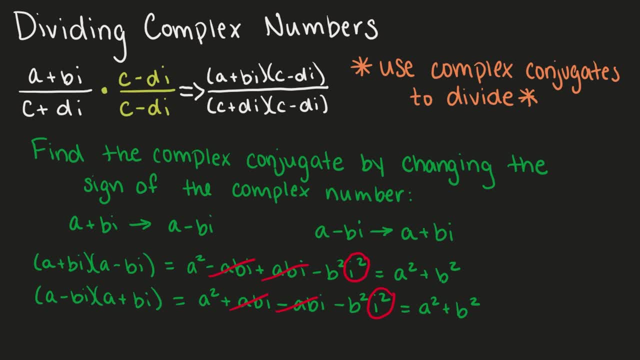 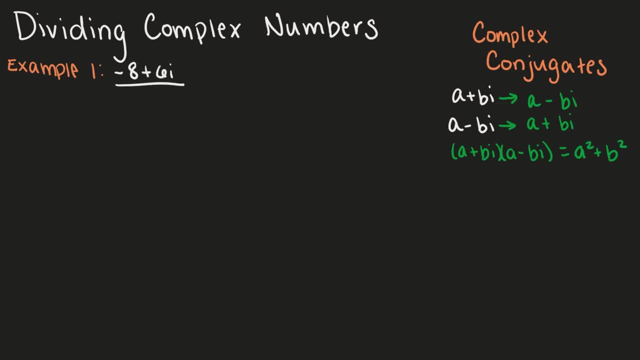 Let's look at this in action. We have negative 8 plus 6i divided by 8 minus 5i. Our complex conjugate is 8 plus 5i. We use the opposite sign of the complex number in our denominator, so 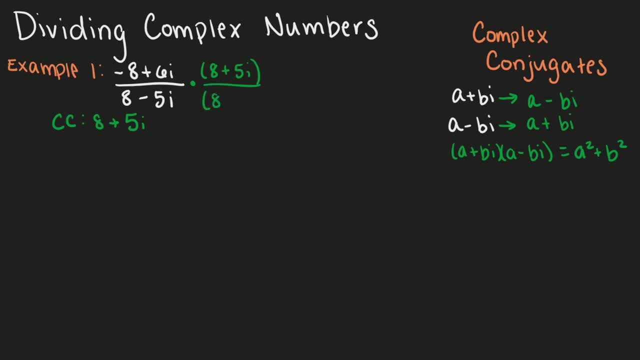 we're going to multiply top and bottom of this fraction by our complex conjugate, which is 8 plus 5i. We can always multiply any fraction by the same number over itself, because 8 plus 5i over 8 plus 5i is equal to 1, so all. 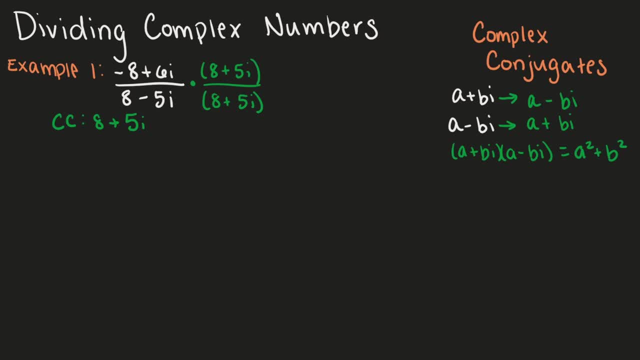 we're doing is multiplying this expression by 1.. This becomes negative 8 plus 6i times 8 plus 5i. over 8 minus 5i times 8 plus 5i. When we FOIL our numerator, we get negative 64 minus 40i plus 48i plus 30i squared. 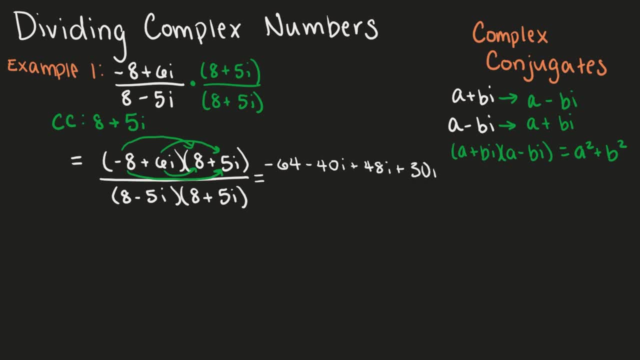 over. remembering our rule. we just need our a and b term, which is eight and five, so our denominator becomes 64 plus 5i. minus 64i is equal to 28.. 25.. i squared is equal to negative 1, so our final answer becomes negative: 94 plus 8i over 89.. 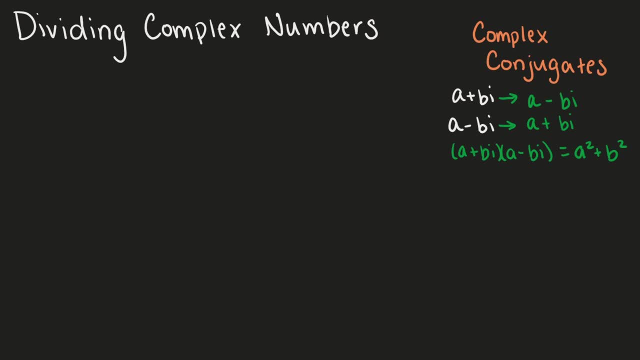 Let's take one more example. We have 10 plus 4i over negative 4 minus 3i. Our complex conjugate is negative 4 plus 3i. The only sign we need to change is in between our real and imaginary. 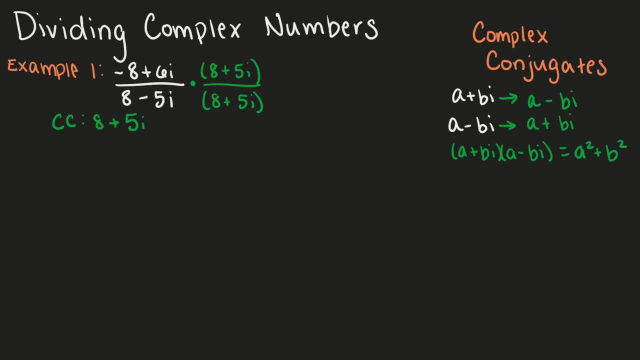 over 8 plus 5i is equal to 1, so all we're doing is multiplying this expression by 1.. This becomes negative 8 plus 6i. times 8 plus 5i over times 8 plus 5i. When we FOIL our numerator, we get: 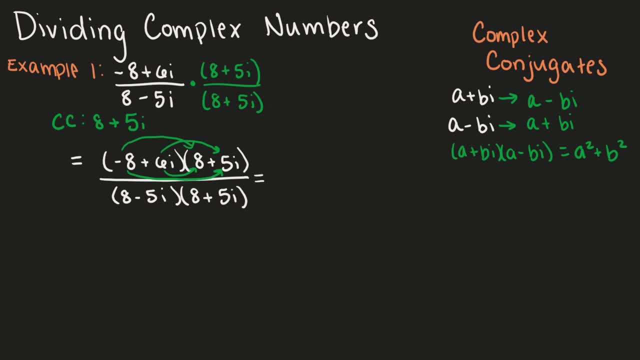 negative: 64 minus 8 plus 5i times 8 plus 5i plus 8 minus 5i. over 8 minus 5i times 8 plus 5i. When we FOIL our numerator, we get minus 40i plus 48i plus 30i squared. 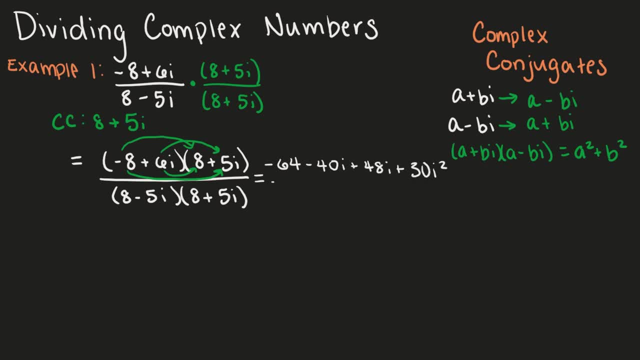 over. remembering our rule, we just need our a and b term, which is eight and five, so our denominator becomes 64 plus 25.. i squared is equal to negative one, so our final answer becomes negative 94 plus 8i over 89.. 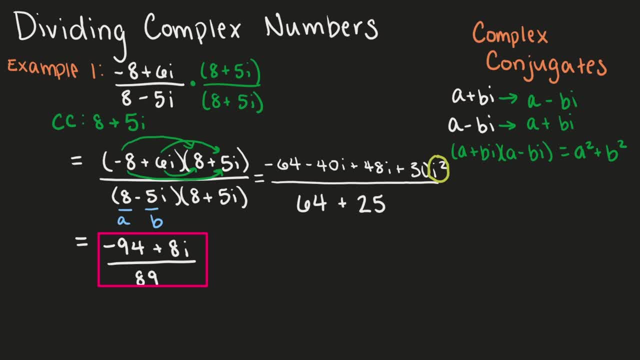 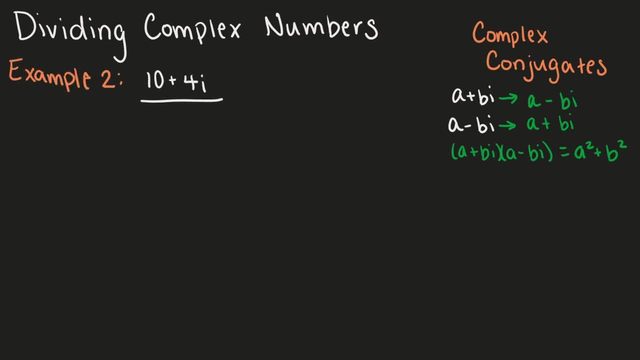 Let's take one more example. We have 10 plus 4i over negative four minus 3i. Our complex conjugate is negative four plus 3i. The only sign we need to change is in between our real and imaginary number. 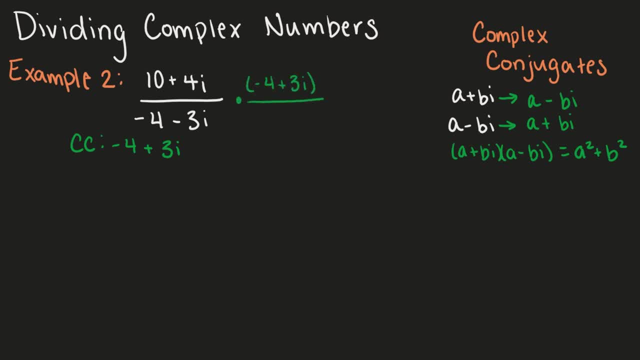 So we're going to multiply our expression by negative four plus 3i over negative four plus 3i. That gives us negative four plus 3i, 10 plus 4i times negative four plus 3i over negative four minus 3i times negative four plus 3i. 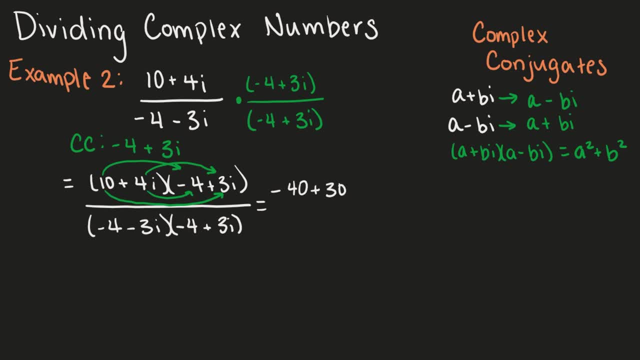 Our numerator becomes negative: 40 plus 30i minus 16i plus 12i squared over. our a is negative four. our b is negative three, so our denominator becomes 16 plus nine. i squared is equal to negative one, so our final answer becomes 52 plus 14i over 25.. 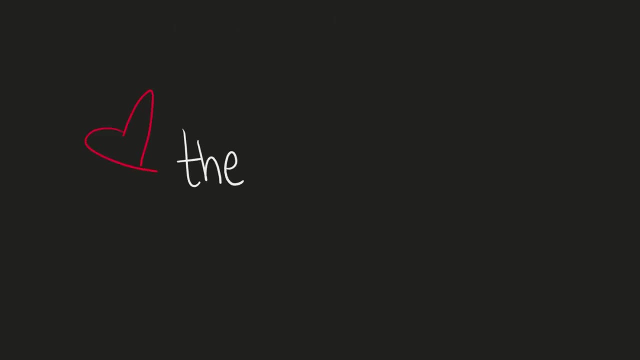 Thank you so much for watching. I hope you enjoyed. Please comment down below what other topics you'd like for me to review. I upload new videos every Tuesday at 1 pm. See you next time.